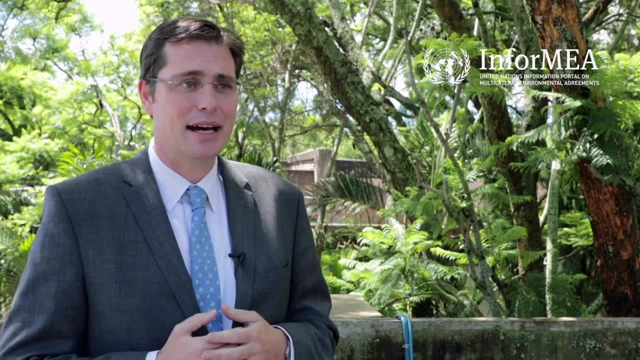 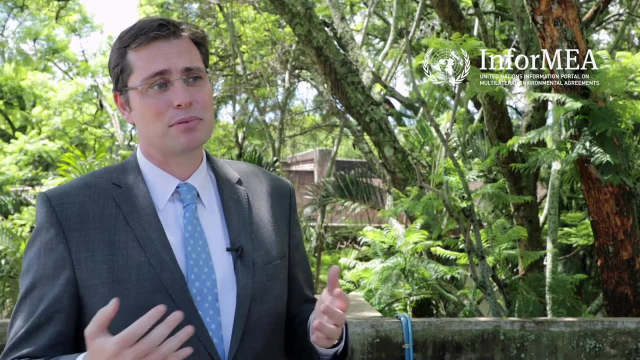 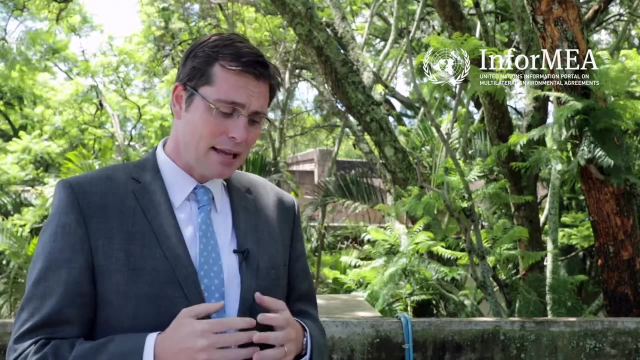 of minutes just to talk about two of the principles in particular. The first, principle 10 of the Rio Declaration. This was a principle, alongside 26 other principles that were decided in the Rio Declaration, which says that environmental issues are best handled when there is public. 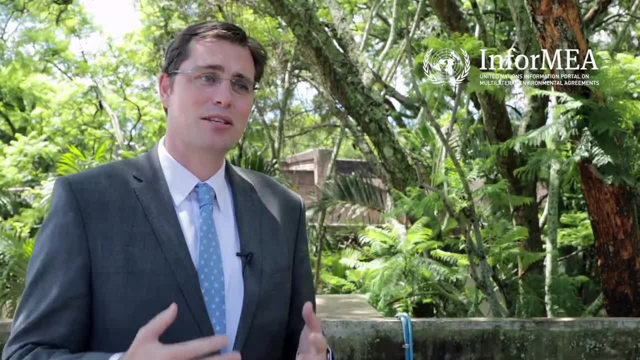 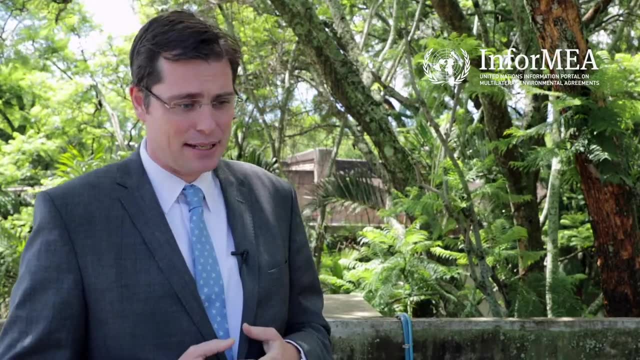 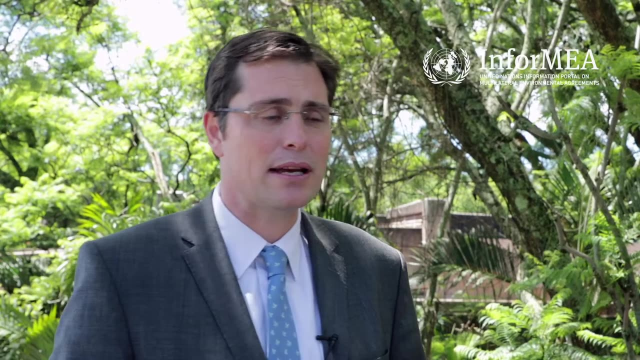 participation when there is access to information and when there are rights to remedies- judicial and administrative remedies. It's a principle that we can see on the international scale, not only through the Rio Declaration, but also taken up by UNEP's governing council. 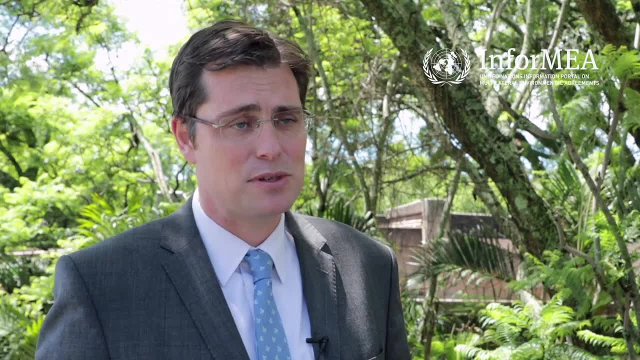 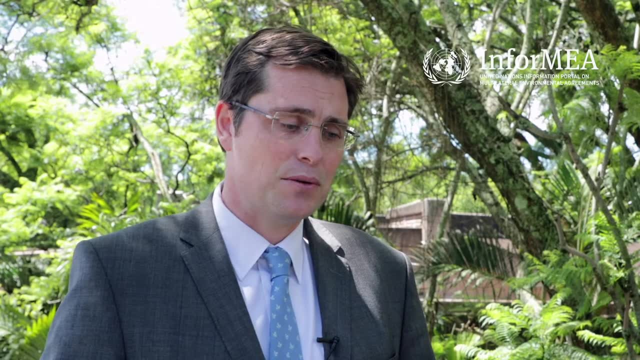 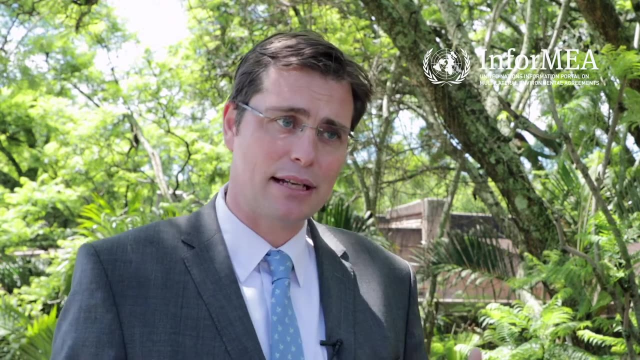 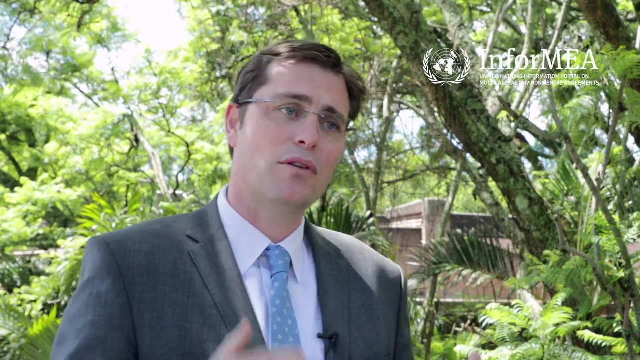 in 2010 through the Bali Guidelines, which further articulated what this principle could mean. We also see principle 10 given legal force through regional legal instruments, Most recently the Escazú Agreement in Latin America and the Caribbean. Before that, we 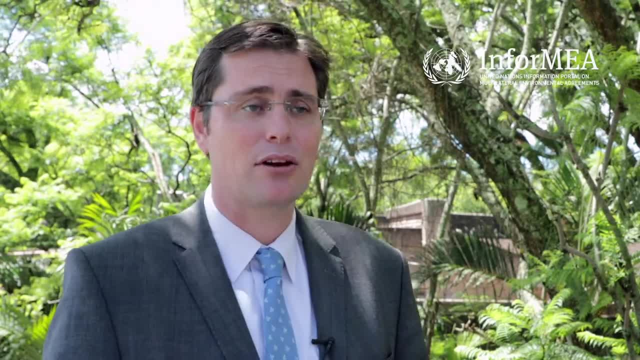 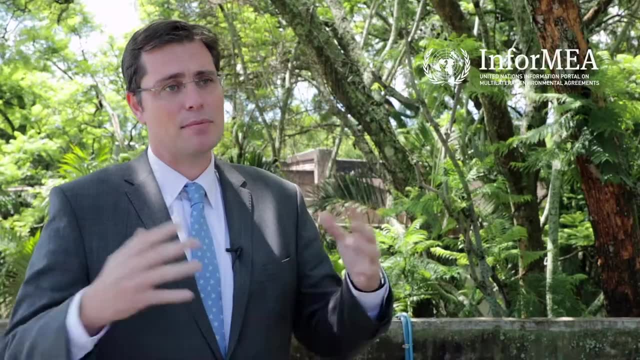 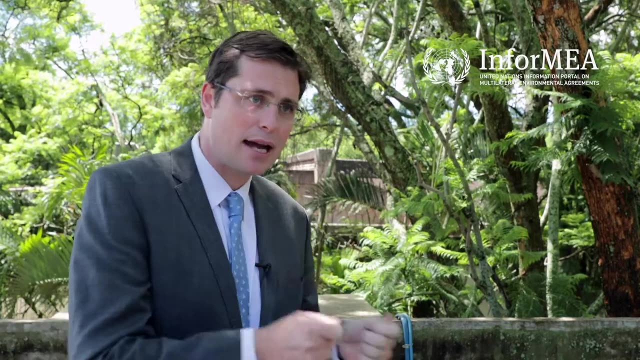 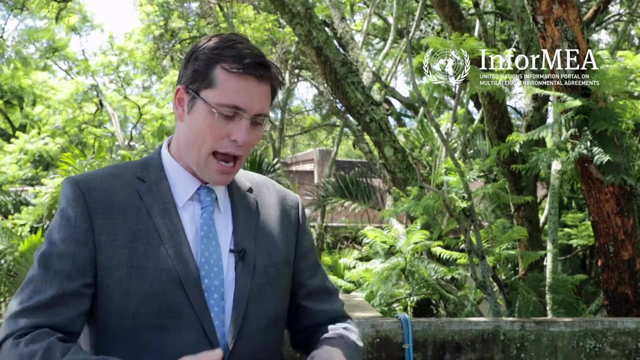 have the Aarhus Convention, technically not a regional agreement, because it is open to all member states to exceed or ratify, But these agreements give legal force to those three core principles of environmental democracy: The right to public participation, the right to information and the right to remedies. At the national level is where we see this. 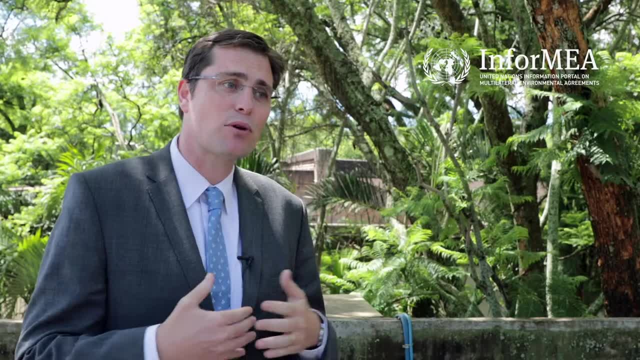 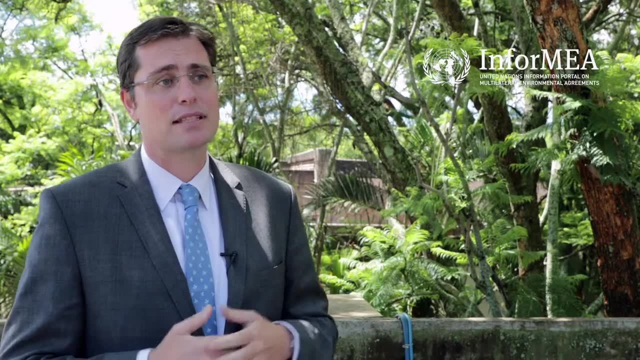 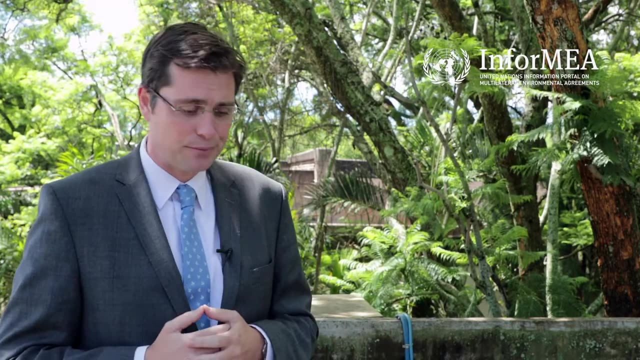 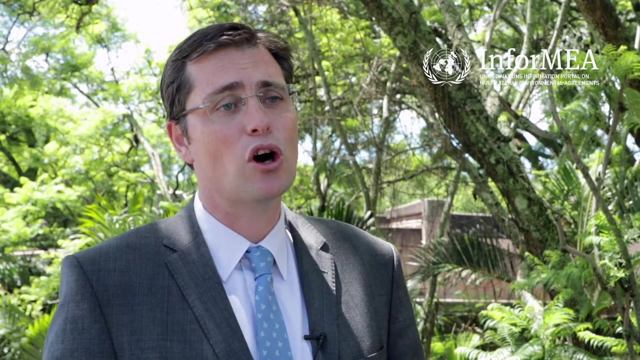 principle really taken up most principally through environmental impact assessment legislation, but also in the decisions of courts, And there are some seminal decisions, including the court in Costa Rica, which gave legal effect to this principle. Another principle that I think is worth mentioning is the idea and principle of non-regression. 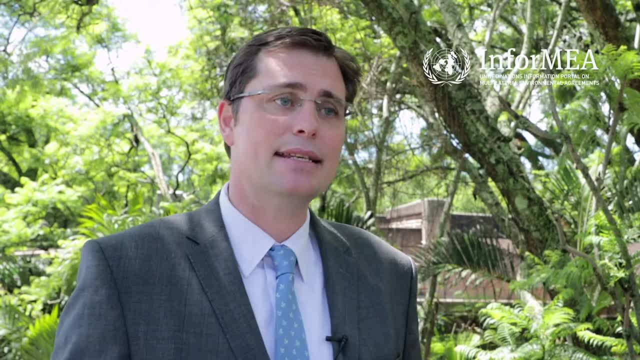 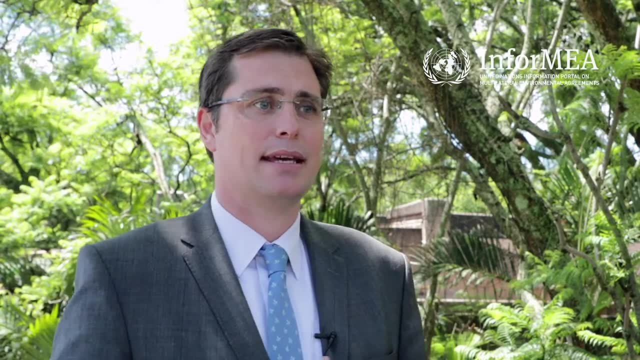 and its cholera progression. This is the idea that environmental laws should not backtrack or backslide. You should not go backwards in the process. You should not go backwards in the process. You should not go backwards in the process. You should not go backwards.